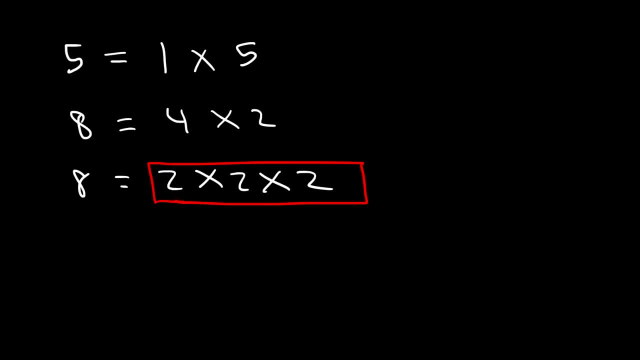 8 if you break it down into a product of its of prime numbers that multiply to 8.. So let me give you another example. 7 is a prime number because 7 is equal to 1 times 7.. Anytime 1 is one of the factors, then this number is a prime number. If we 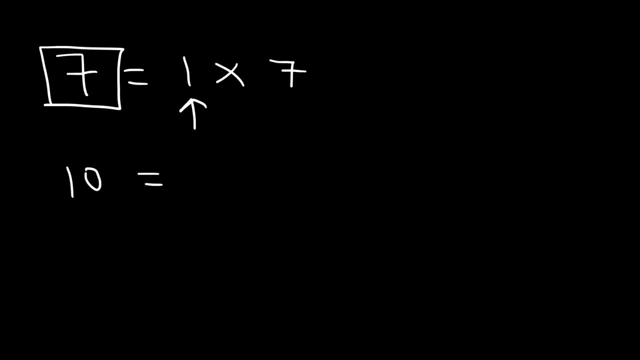 take 10,. 10 can be broken down into two prime numbers, one of which is not 1.. So 10, you could write it as 2 times 5.. If you can break it down into prime numbers that don't contain 1,, then this original number, 10, is a composite number. 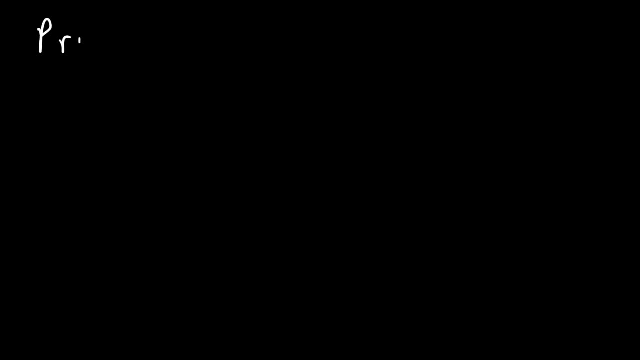 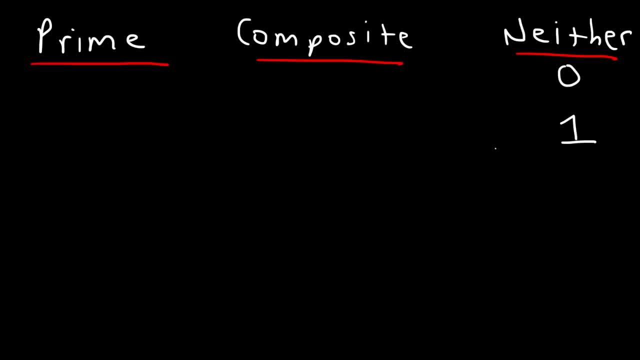 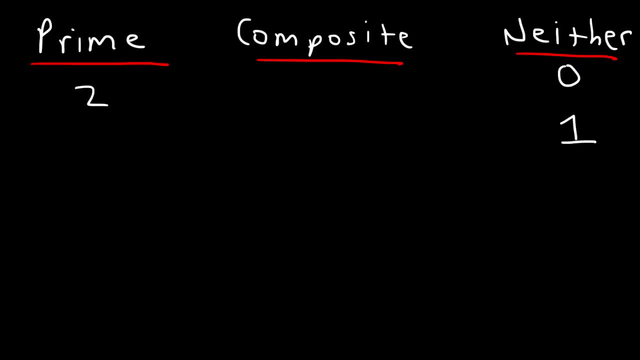 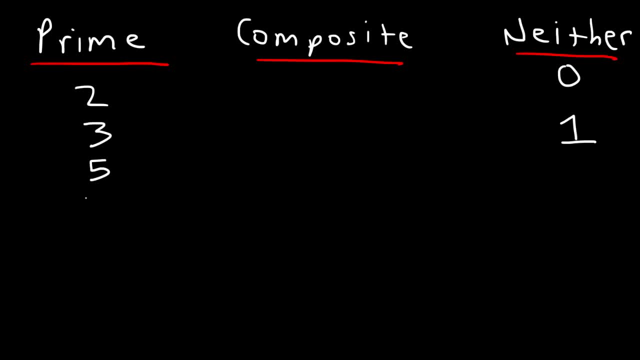 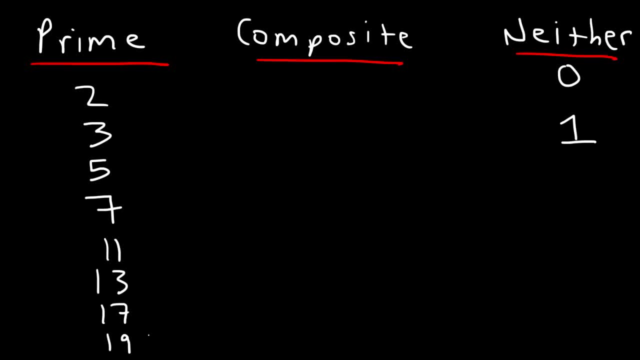 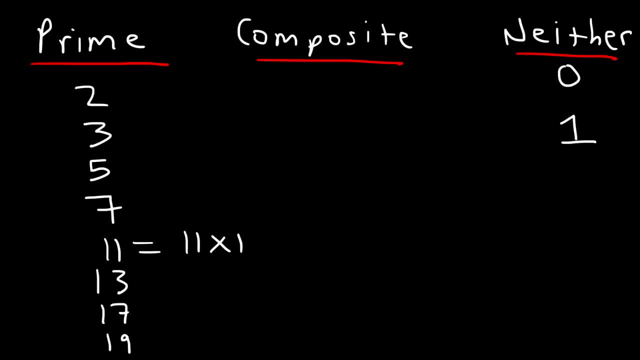 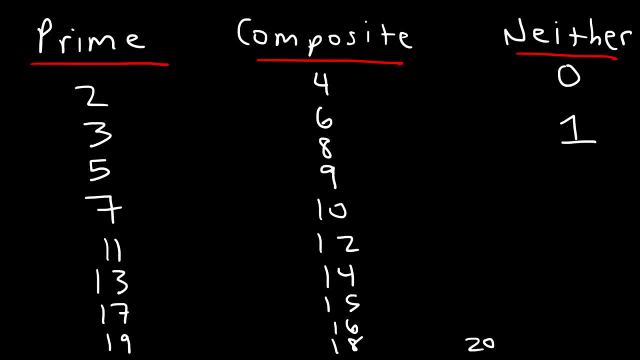 composite numbers can be written as a product of factors that doesn't include 1.. So 4 can be written as 2 times 2.. That's the prime factorization of 4.. 6 can be written as 3 times 2.. As you can see, you can break it down into small. 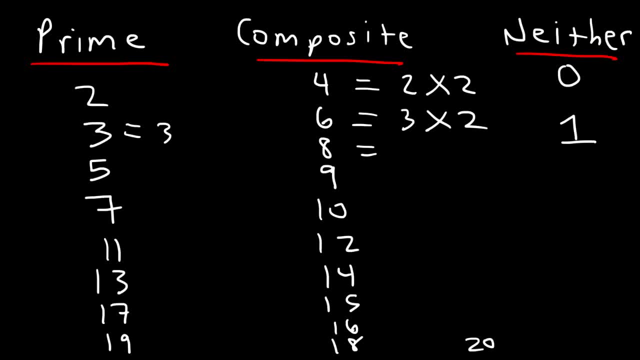 numbers that doesn't include 1.. If it does include 1, then it will be a prime number. All the prime numbers will have 1 as a factor, and that's the key difference that separates prime numbers from composite numbers. 8, we said it's 2. 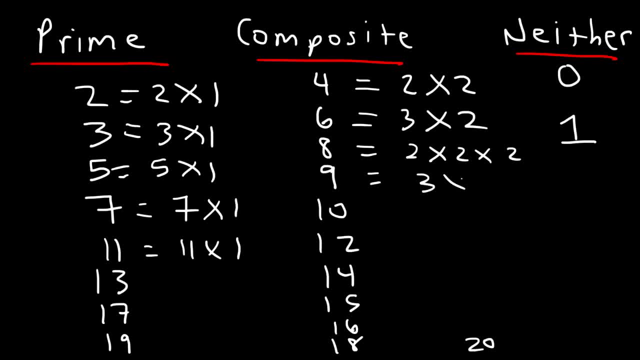 times 2 times 2.. 9, you can write it as 3 times 3.. 10 is 5 times 2.. 12, it's 3 times 4, and 4 can be broken down into 2 times 2.. 14 is 7 times 2.. 15 is 5 times 3, and you get the. 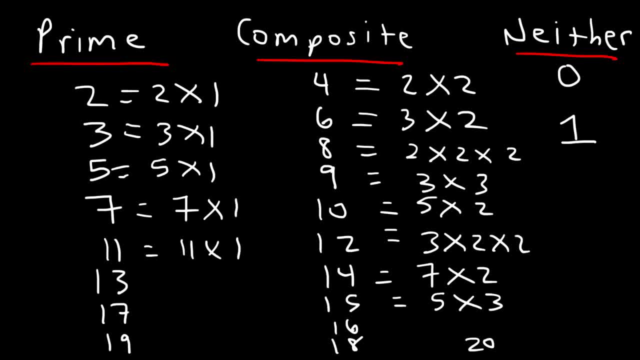 point. All of the composite numbers can be broken down into prime numbers that don't contain 1.. All the prime numbers can be broken down into factors. where 1 is included, It's going to be 1 times itself. That makes it prime And just. 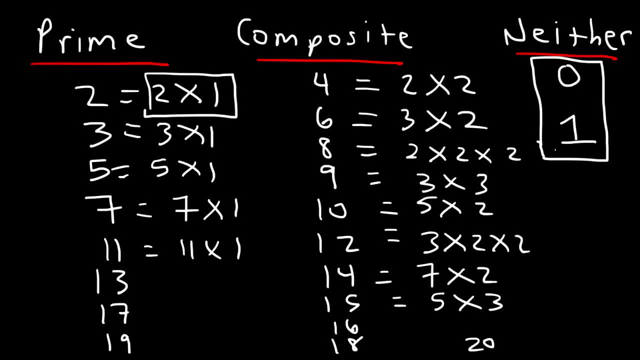 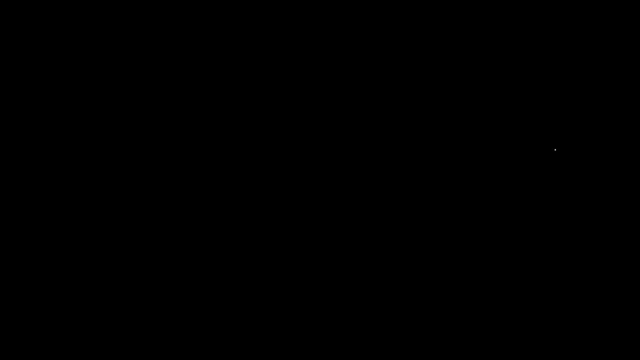 remember, 0 and 1 are considered not to be prime or composite numbers. Now let's talk about writing the prime factorization of larger numbers. What is the prime factorization of 50?? Now you can use the factor tree to help you out in this case. So first let's divide 50 by the smallest prime number. 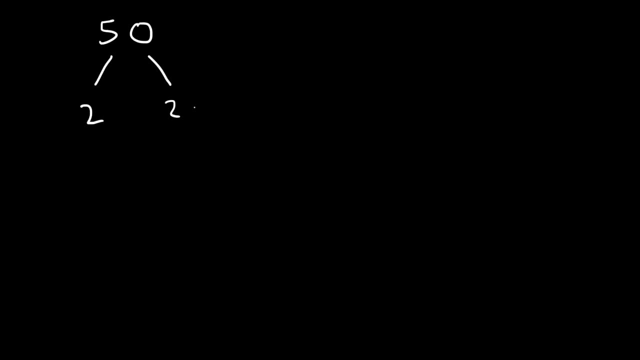 that we know of, which is 2.. 50 divided by 2 is 25.. Now, once you have a prime number, we want to write 50 by detective meaning 50 times 50, because the 5- reunited numbers are functions. so if you didn't get the prime factorization on 50,. 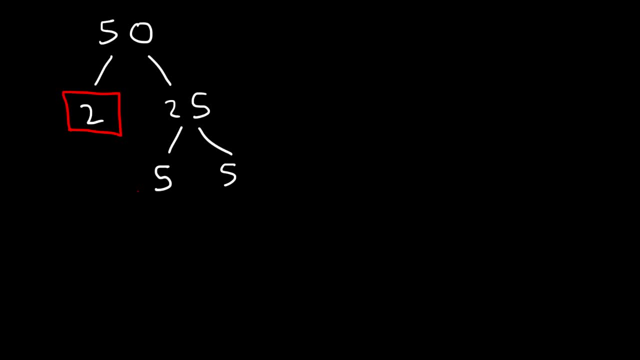 you wouldn't really want to highlight it or circle it, because you're going to use that when writing the prime factorization of 50.. 25 is a composite number and you could break it down into 5 times 5,, both of which are prime. 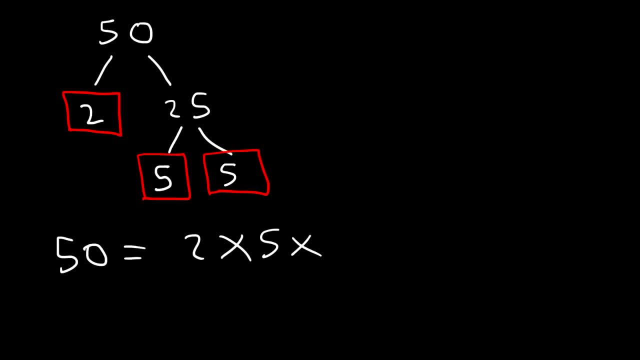 numbers. When you have no more composite numbers, then you can make a list, as a product of the factors, of all the prime numbers that compose it. Now, sometimes in your homework you may be asked to write the prime factorization using exponents. 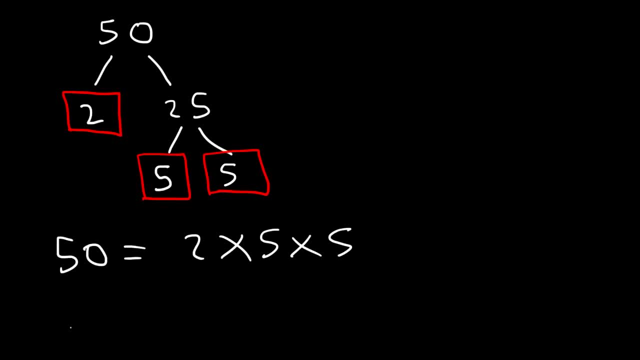 Because we have two 5s, we can write it as 5 squared. So you can express the prime factorization of 50 like this: You could say: it's 2 times 5 squared, since we have two 5s. 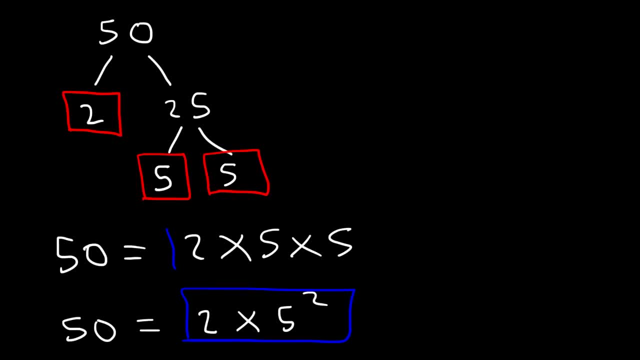 So you can leave the answer like this, or you can write it this way, But for the sake of practice I'm going to write it both ways. So now it's your turn. Write the prime factorization of 120.. Feel free to pause the video. 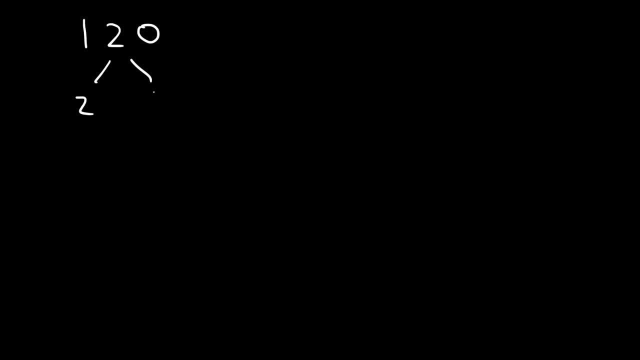 So first let's divide 120 by 2.. 120 divided by 2 is 60.. Now, 60 is an even number, which means that it's divisible by 2.. 60 divided by 2 is 30.. 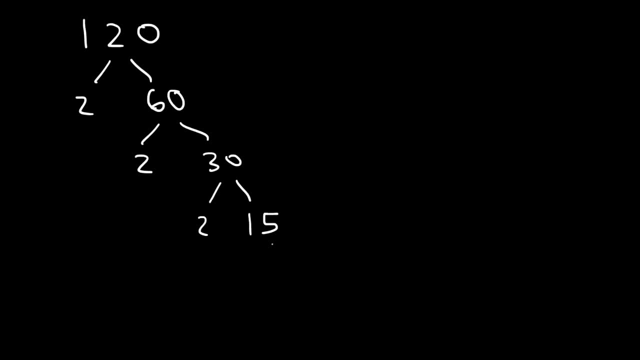 30 is also an even number, so let's divide it by 2. That's going to give us 15. And 15.. 15 is a composite number that we're familiar with. It's 5 times 3.. So these are all the prime numbers. 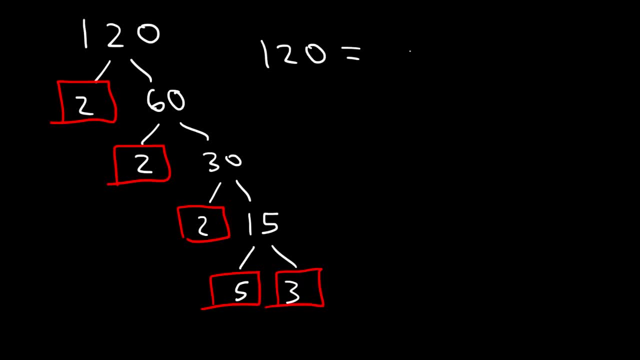 So 120 is 2 times 2 times 2 times 3 times 5, in ascendant order. Now to write it using exponents, we're going to simplify it. These three 2s, we're going to write it as 2 to the 3rd power. 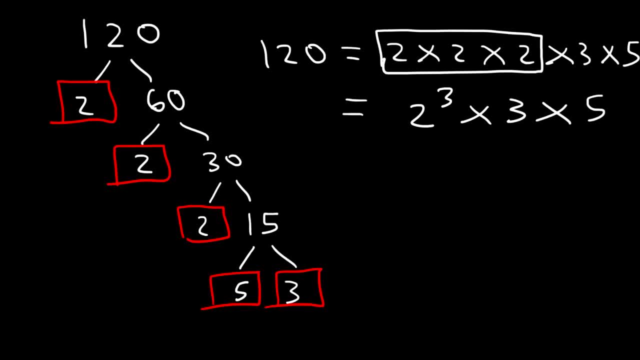 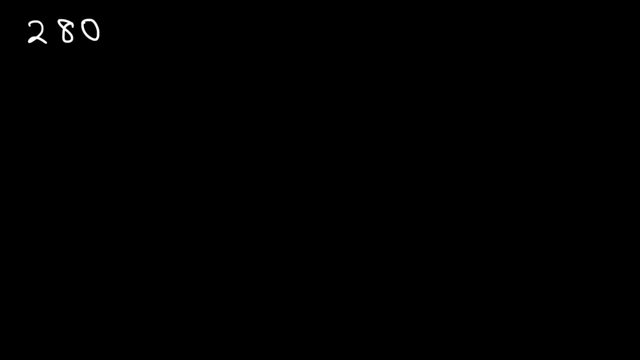 and then times 3, times 5.. So that's the prime factorization of 120 using exponents. Now let's work on another example. Let's write the prime factorization of 280.. So feel free to pause the video if you want to try it. 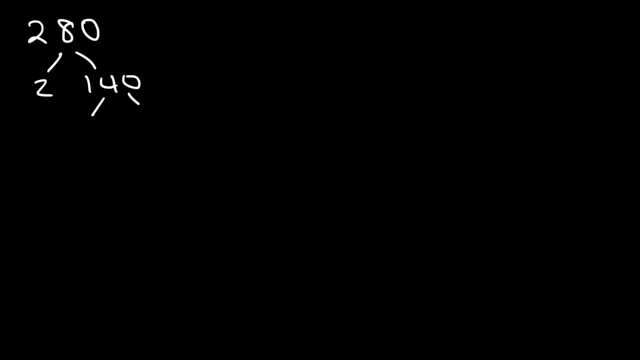 So 280 divided by 2 is 140.. And if we divide it by 2, that will give us 70.. And if we divide 70 by 2, that's 35.. 35 has a 5 at the end, so it's divisible by 5.. 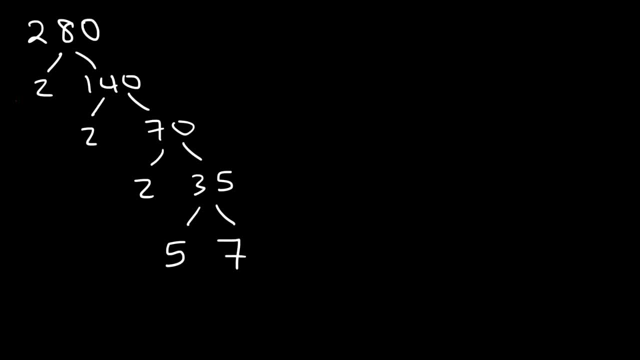 35 divided by 5 is 7.. So these are the prime numbers that compose 280. Or 280 consists of those prime numbers. So 280 is 2 times 2 times 2 times 5 times 7.. So we can write it as 2 to the 3rd power. 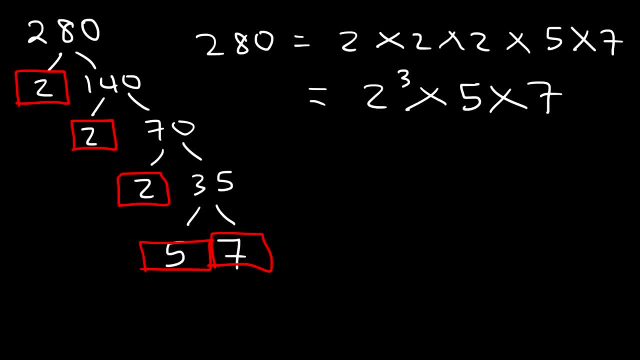 times 5 times 7.. Here's another one that you can work on for the sake of practice: 540.. Go ahead and write the prime factorization of 540 using the factor tree method. So since it has a 0 in front, we know it's even. 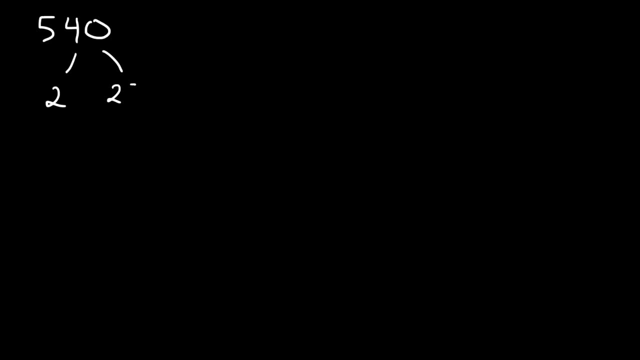 Let's divide it by 2.. 540 divided by 2 is 270.. And then we can divide that by 2.. That's going to be 135.. Now, 135 is not an even number, It's an odd number. 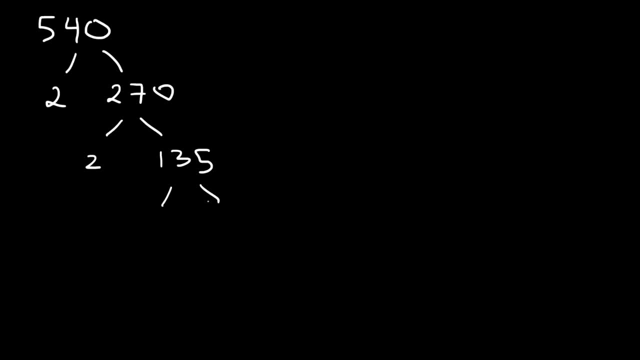 And it ends in 5, so we can divide that by 5.. So 135 divided by 5 is 27.. 27- we could divide it by 3.. 27 divided by 3 is 9.. And 9 divided by 3 is 3.. 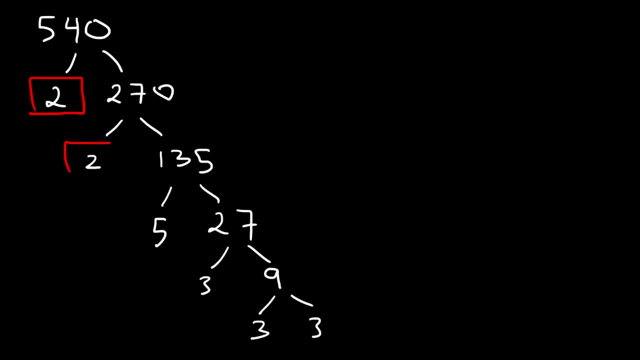 So 9 is 3 times 3.. So these are all the prime numbers that multiply To 540.. So to write it in ascending order, we can say that 540 is 2 times 2 times 3 times 3 times 3 times 5.. 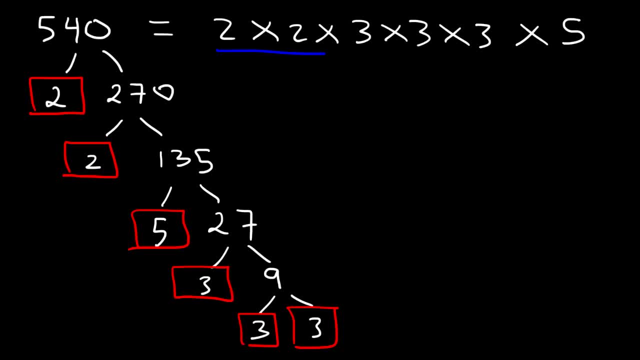 So now let's write it using exponents. So we have two 2s, So we can write 540 as 2 squared times. And then there are three 3s, So times 3 to the 3rd power and then times 5.. 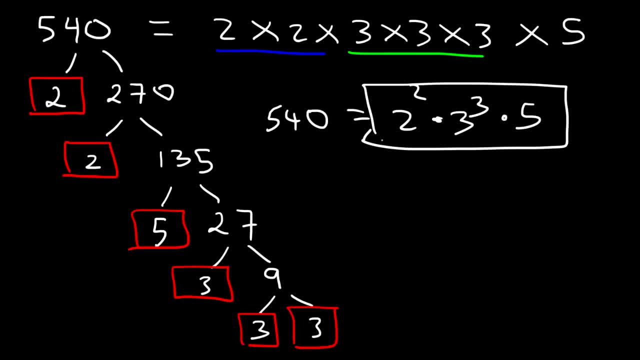 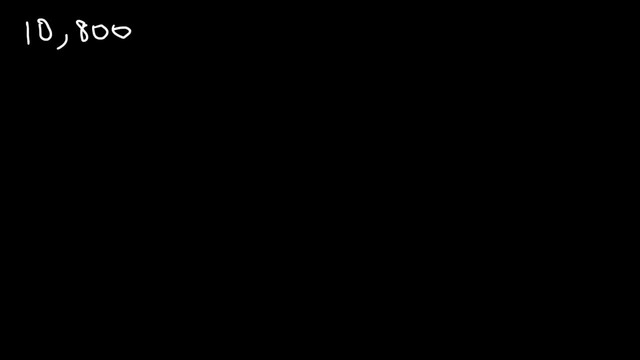 So this is the prime factorization of 540 using exponents. Here's another example. It's a much larger number, 10,800.. Go ahead and try that one. So this might take some more work. Let's divide it by 2.. 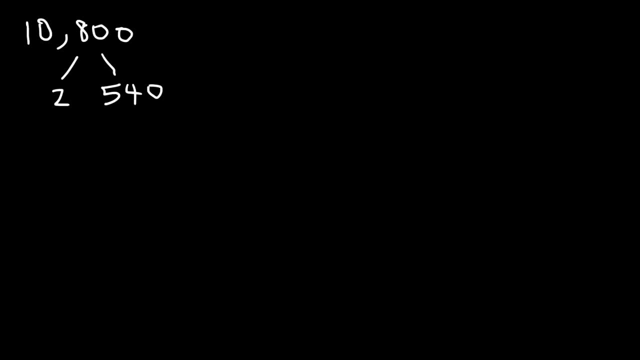 Half of 10 is 5.. Half of 8 is 4.. So half of 10,800 is 5,400.. If we divide it by 2,, 54 divided by 2 is 27.. So this is going to be 2,700.. 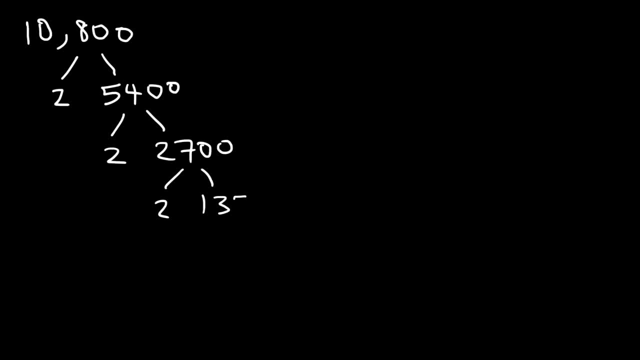 And then, if we divide that by 2, this is going to be 1,350.. And we could divide 1,350 by 2 due to the 0 at the end, And that's going to be 675.. Now this ends with a 5.. 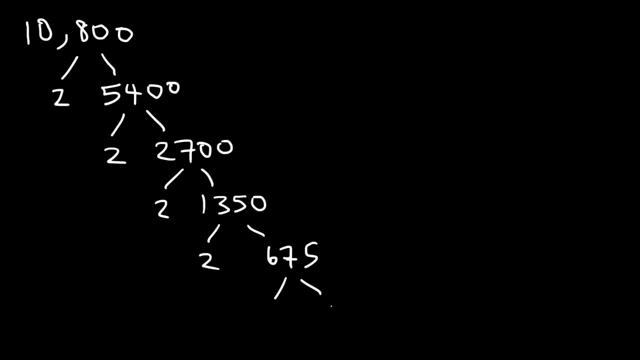 So that means it's divisible by 5.. It's no longer even, so chances are it won't be divisible by 2 anymore. If we divide it by 5, 675 divided by 2, 5 is 135.. So there's another 5.. 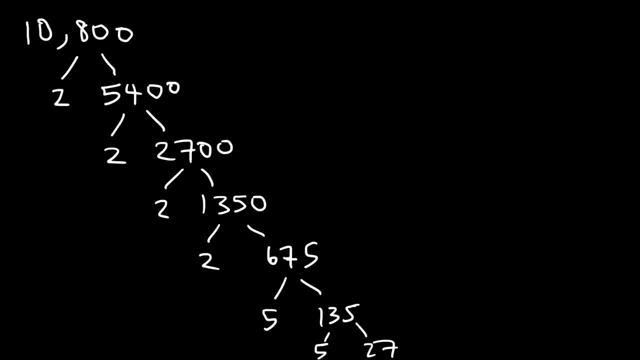 135 divided by 5 is 27.. Now let me just continue this here. 27 is 3 times 9.. And 9 is 3 times 3.. So let's box in all of the prime numbers that we have.